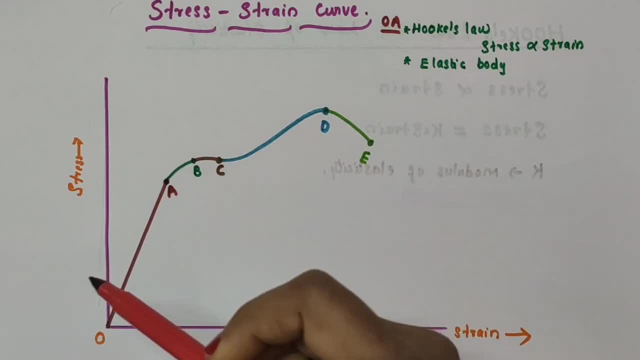 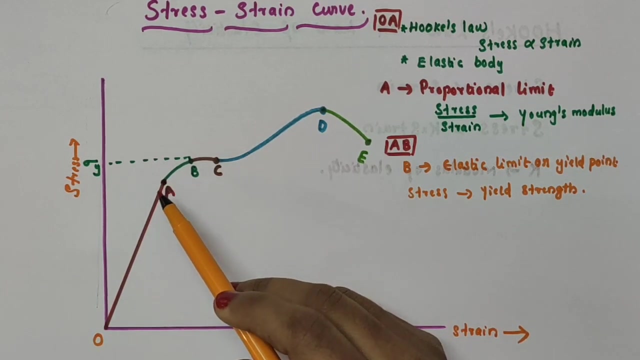 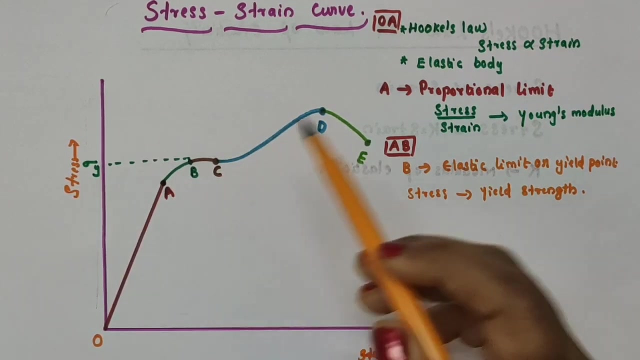 that is, shape, size, etc. when the applied force is removed, That is, a solid behaves as an elastic body. in this region between O and A- See this point A- this is actually called as proportional limit, Because in this limit stress will be proportional to strain and stress by strain ratio. 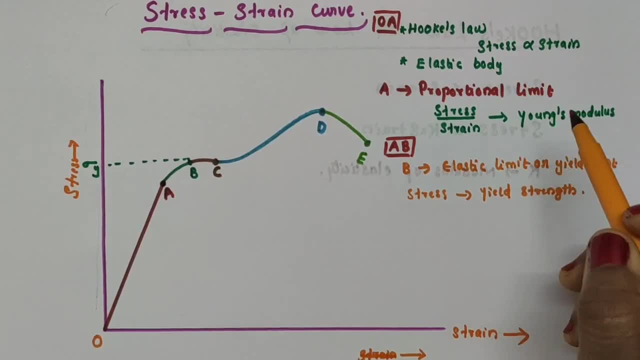 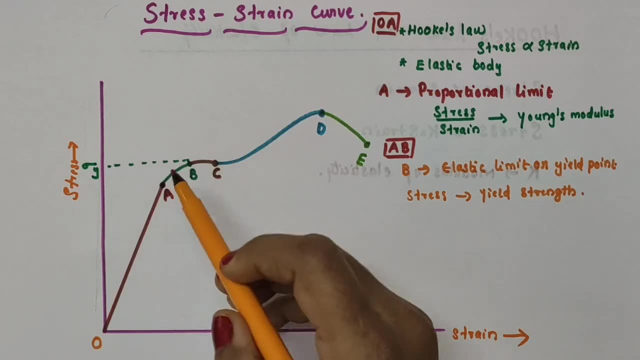 that gives us a proportionality constant, which is known as Young's modulus, which we will discuss in our next video. Anyway, I will provide the link for that in the description box. Next, consider this region AB. Okay, we are considering this region AB now. 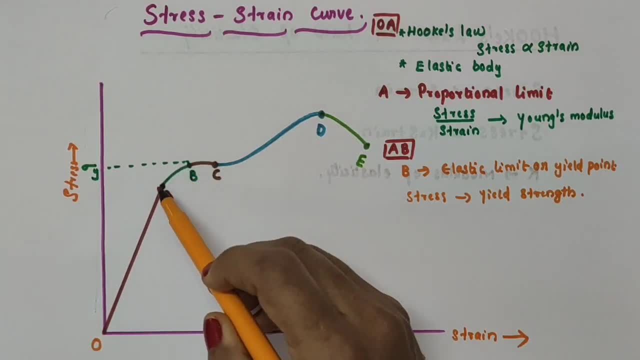 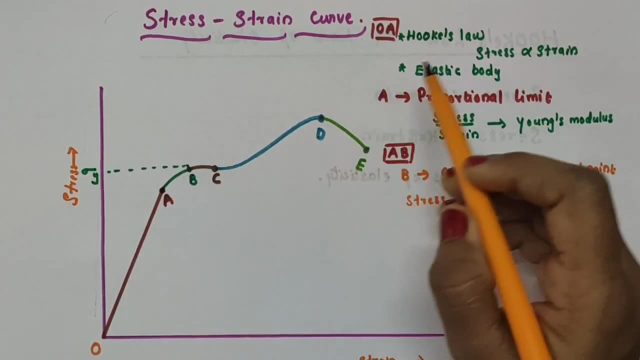 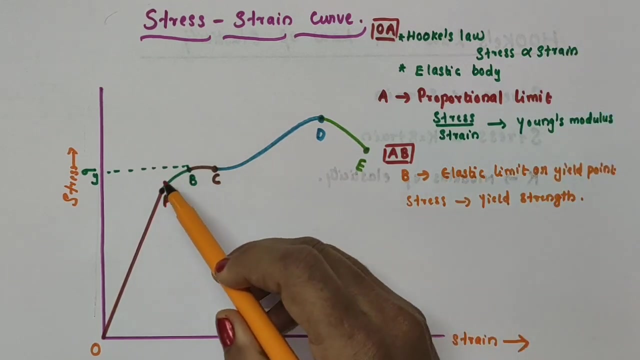 That is the region between A and B. In this region from A to B, you can see that the curve is not a straight line here. So in this region stress is not directly proportional to strain. That is, stress and strain are not directly proportional because this is not a straight line. 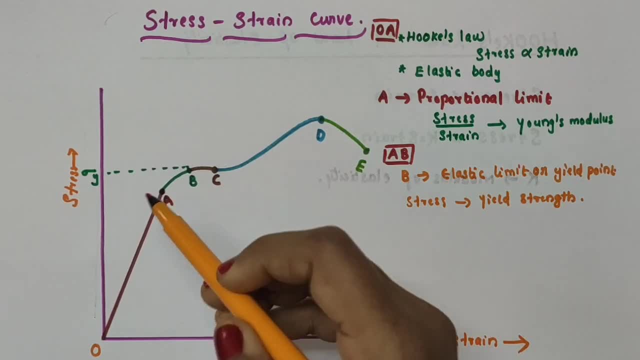 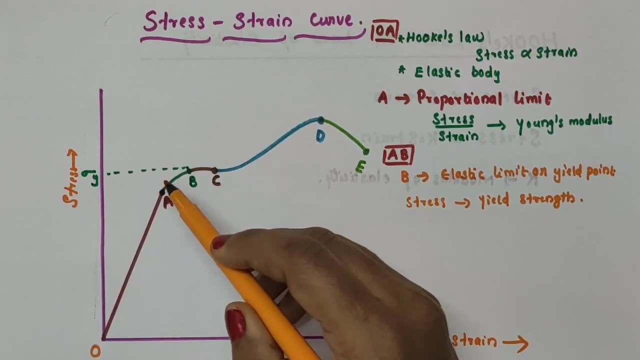 However, the body still returns to its original dimension when the load is removed. So in this region the stress and strain are not proportional, But the body has that elastic property by which it returns to its original dimension when the load or applied force is removed. 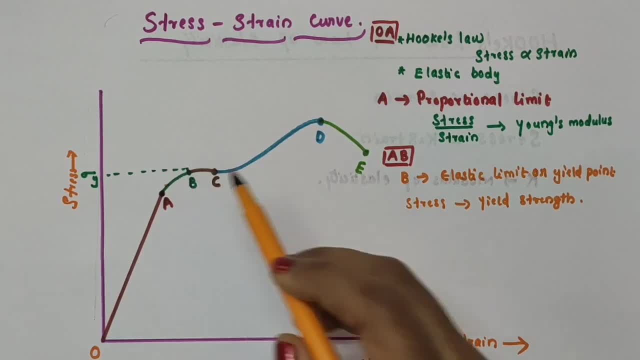 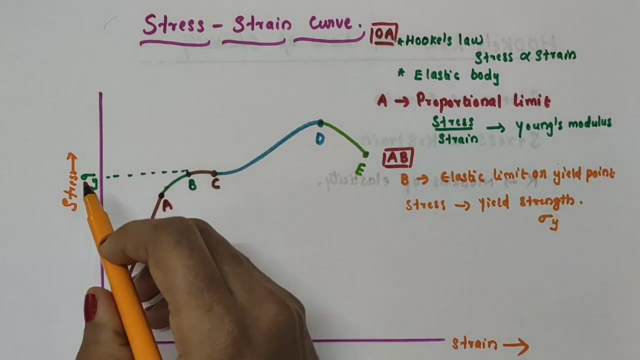 So this point B, it is actually known as elastic limit or yield point. The corresponding stress is actually called as yield strength and it is represented by sigma y. Okay, yield strength of a material is represented by sigma y, So the stress corresponding to this point that is actually called as: 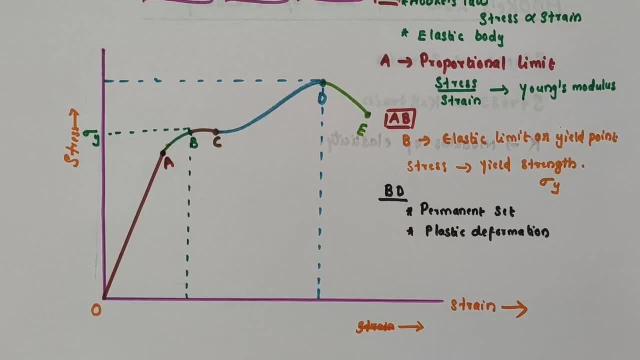 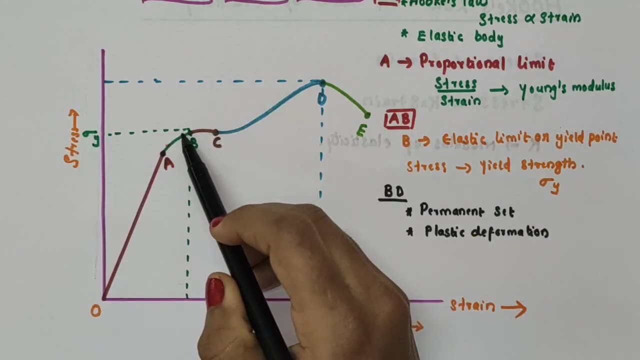 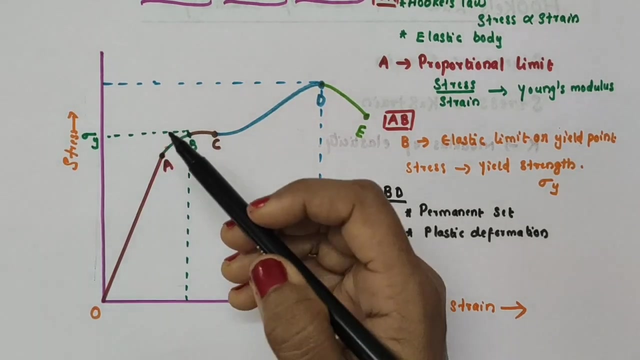 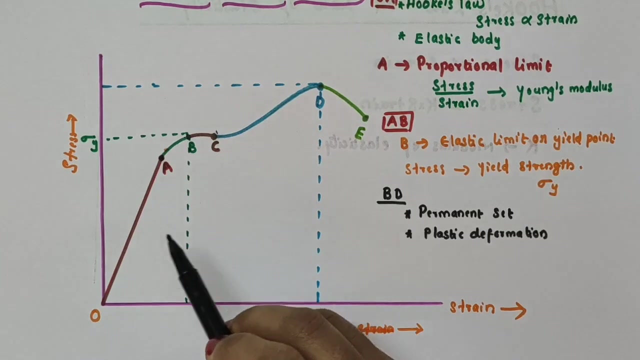 yield strength: sigma y. So this point B is called as elastic limit, because this is the point in the graph or curve up to which the material or body can return to its original dimension when the load is removed. Beyond this point or beyond this limit, the body does not return to its original dimension. 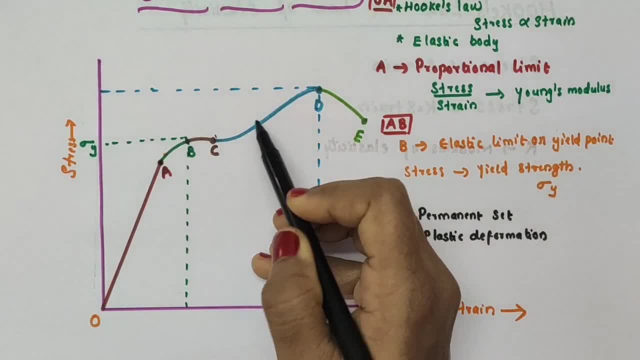 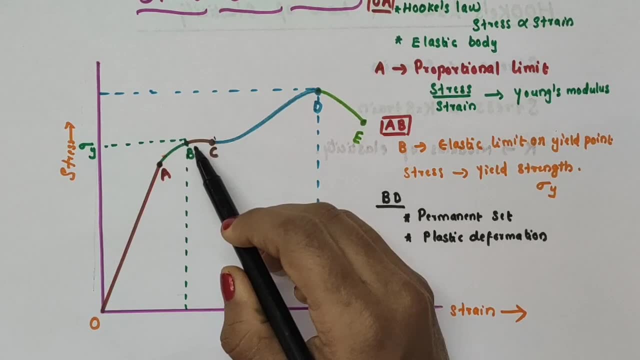 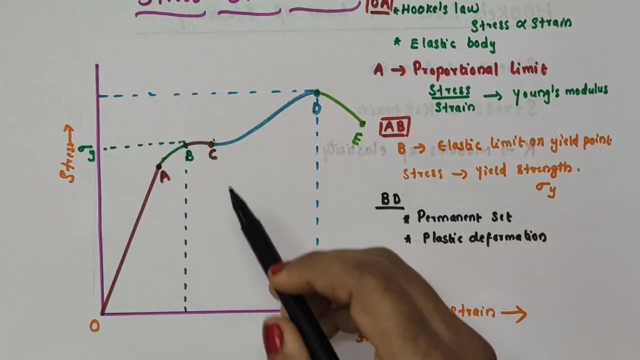 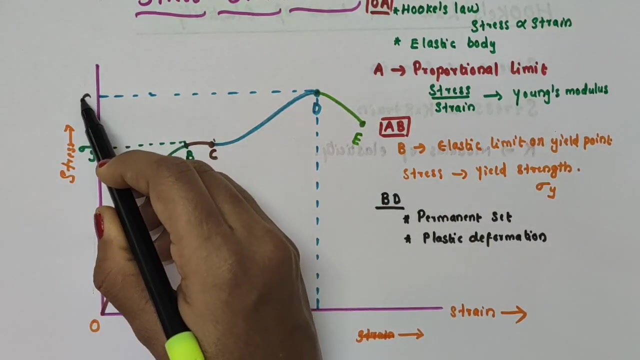 Okay. now if the load is increased further, the stress developed exceeds this yield strength sigma y. And even for a small change in the stress the strain increases rapidly. This portion of the curve, actually BD, shows that. See, from B to D, the change in stress is only this much. 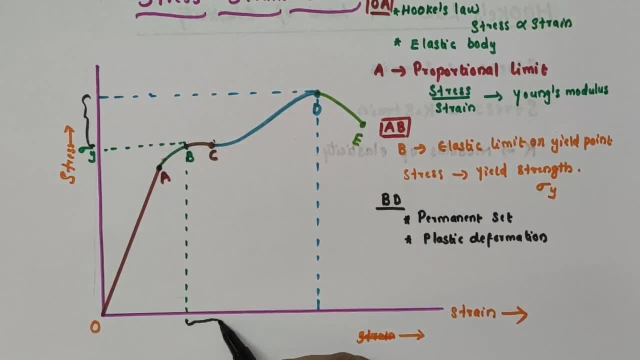 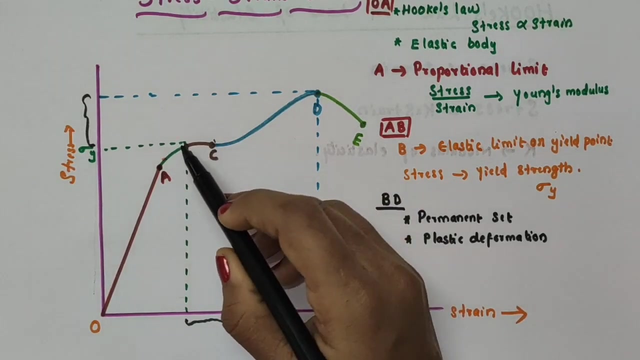 Okay, but you see the change in stress, The strain change in strain is this much? no, Okay. so for a small change in stress, the strain increased rapidly. no, Okay. now consider a point C, between B and to D. 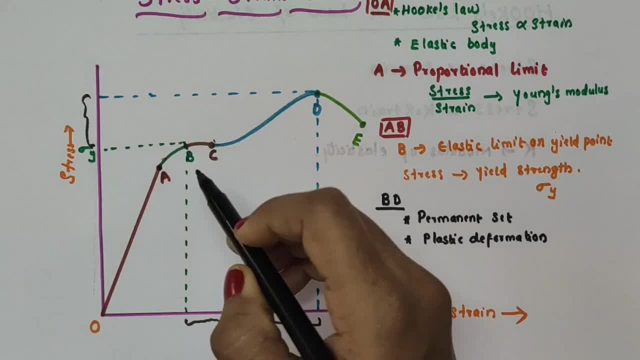 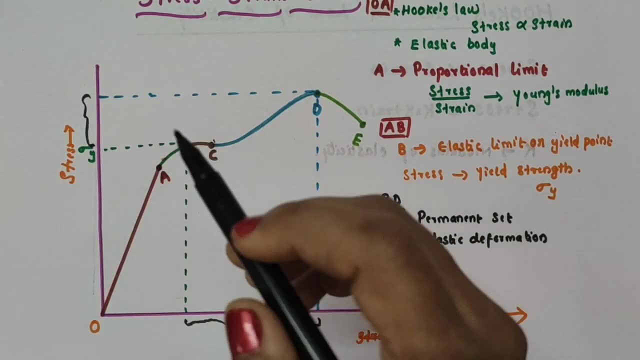 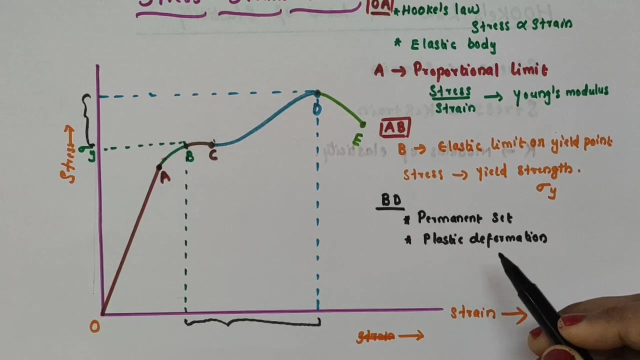 At this point C, when the load or applied force is removed, the body does not regain its original dimension. That is, the material is said to have a permittivity. That is, the material is said to have a permanent set. The deformation is said to be plastic deformation. 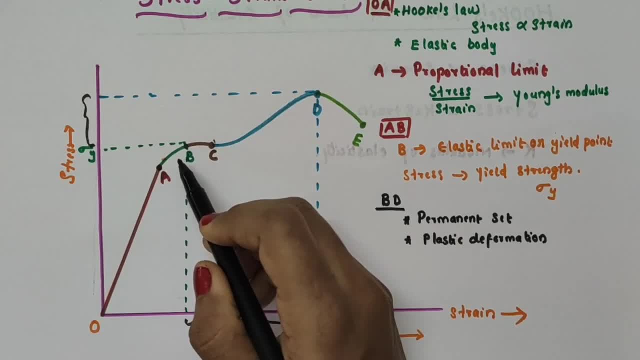 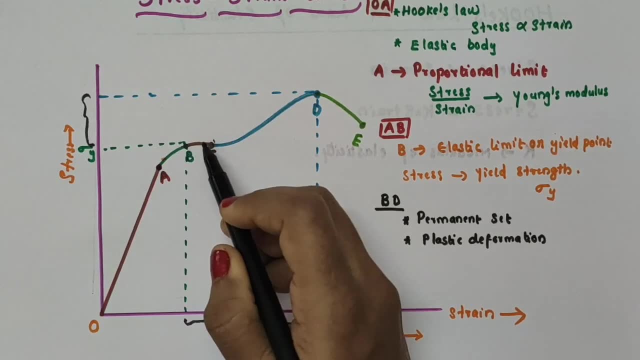 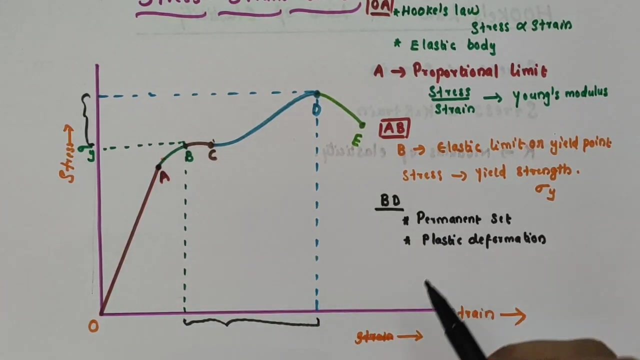 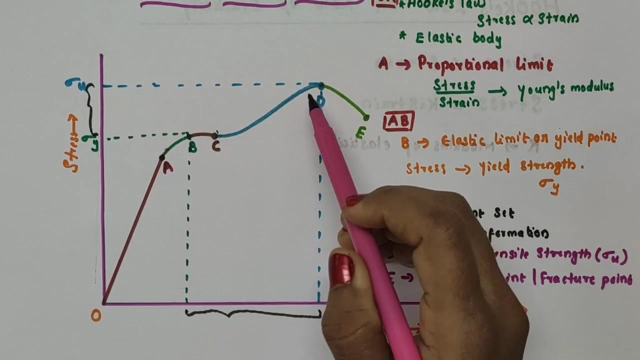 That is this yield point. no, Okay, it is the point at which the material starts to deform plastically. That is, when this yield point is passed or crossed, permanent deformation of the material occurs. Now, see this point D on the graph. 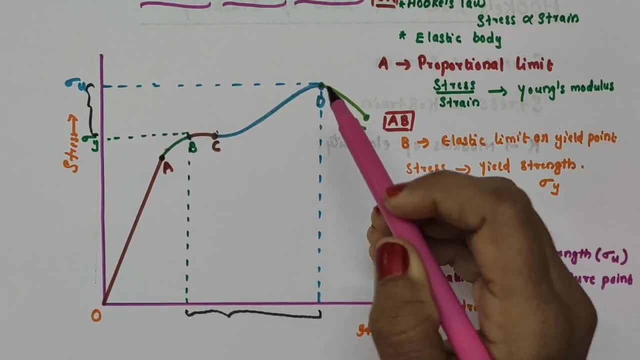 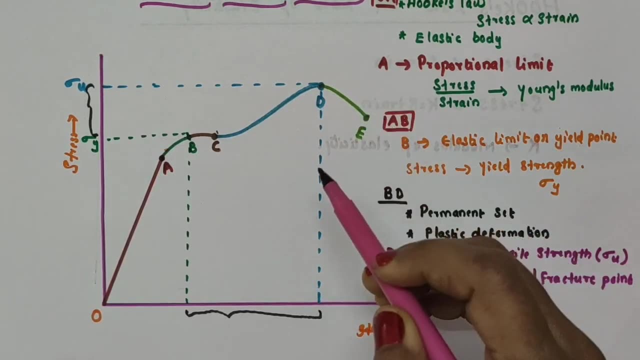 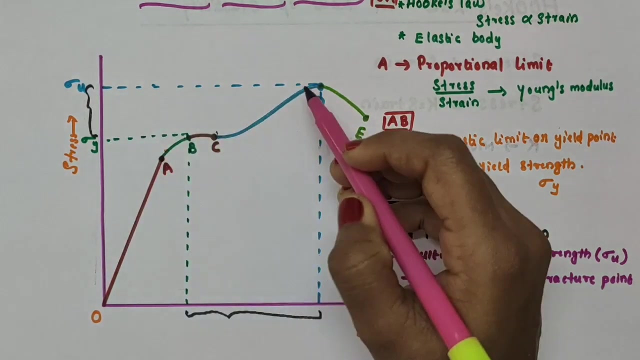 Actually represents the maximum stress that a material can bear or endure before it's breaking. Beyond this point, the material is likely to get broken easily. So this point D on the graph is the ultimate tensile strength, sigma U of the material. 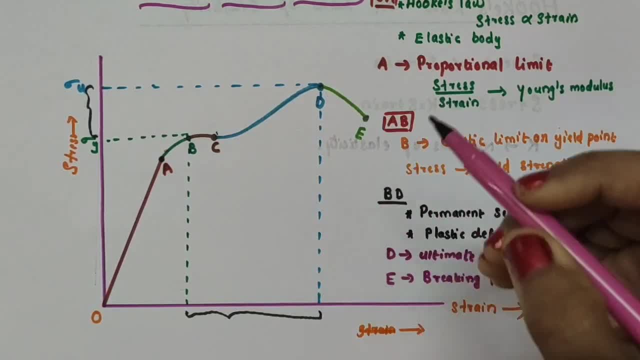 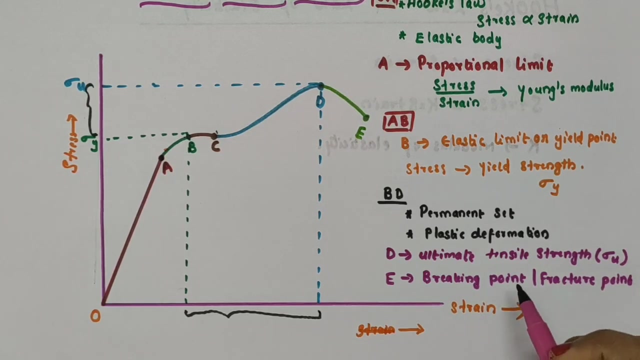 Beyond this point D, additional strain is produced, even by a small- I mean even by a reduced- applied stress And fracture occurs. Occurs at this point E. This point E is actually the breaking point or fracture point. This is the point at which the failure of the material or breaking of the material takes place. 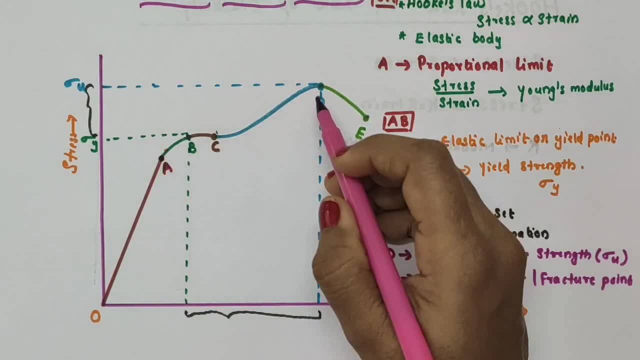 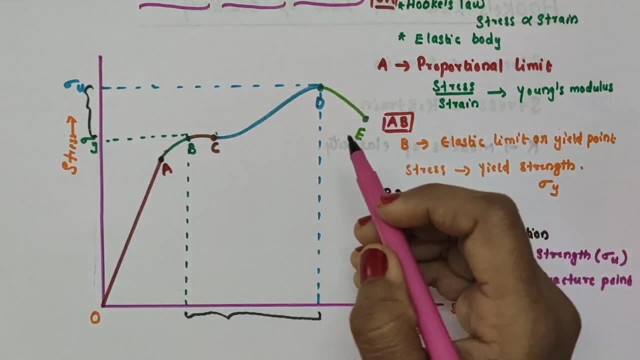 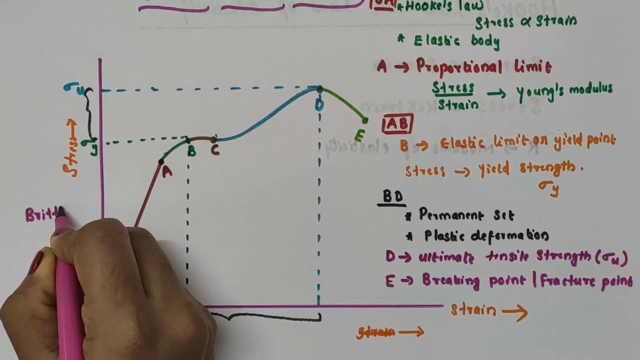 Okay. now, if the ultimate strength, point D, and the fracture, point E, are close, then the material is said to be brittle. Okay, I'm writing here. the material is said to be brittle. Okay, examples for brittle materials are glass, ceramic, etc. 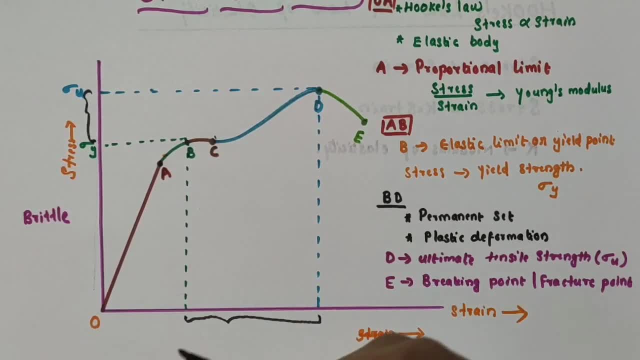 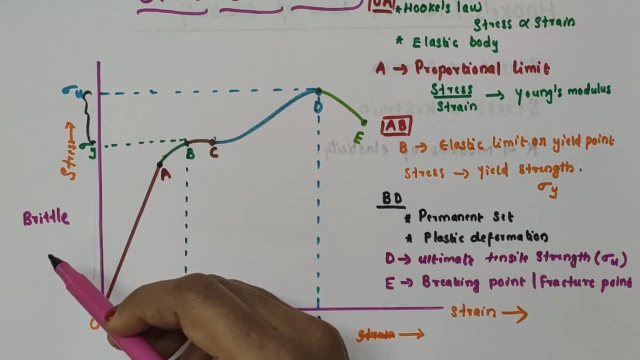 They have extremely low plasticity. that is the cracking of the material can initiate without plastic deformation. That is when a brittle material is subjected to a stress, it breaks with little elastic deformation and without significant plastic deformation It's breaking. The breaking is often accompanied by a snapping sound. 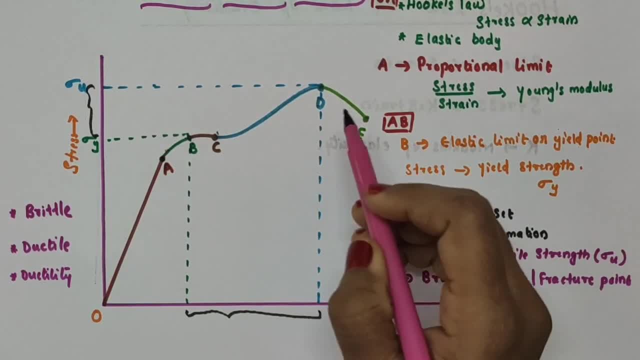 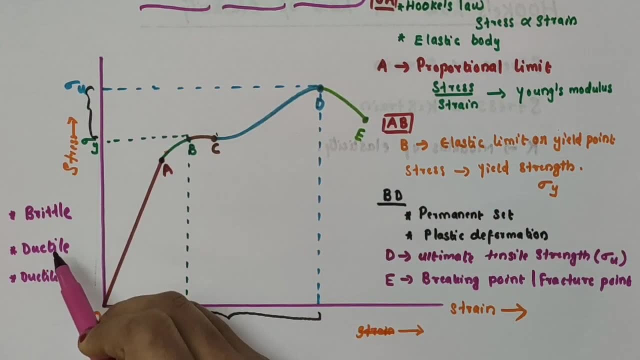 If this ultimate strength, point D, and the fracture point E are far apart, the material is said to be ductile. Examples for ductiles- I mean ductile materials- are steel, aluminum, copper, etc. Ductility is actually the ability of a material to get deformed without fracture. 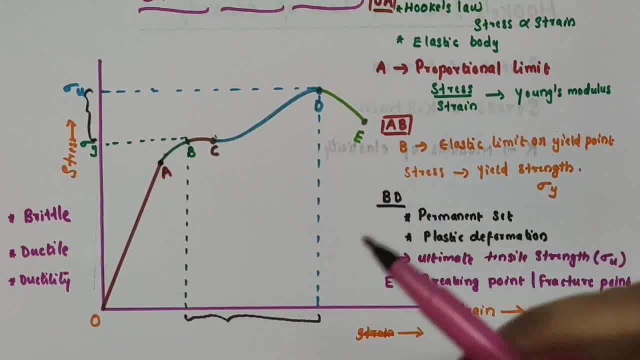 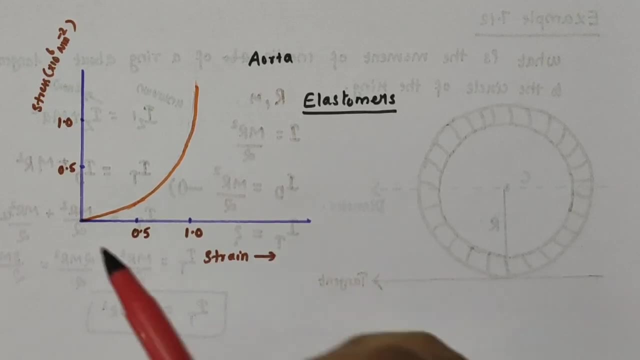 They can be easily stretched. They can be easily stretched into a wire or any other kind of deformations under tensile stress- I mean under actually tensile stress- without breaking. So we have discussed about the typical stress-strain curve for a metal sofa. 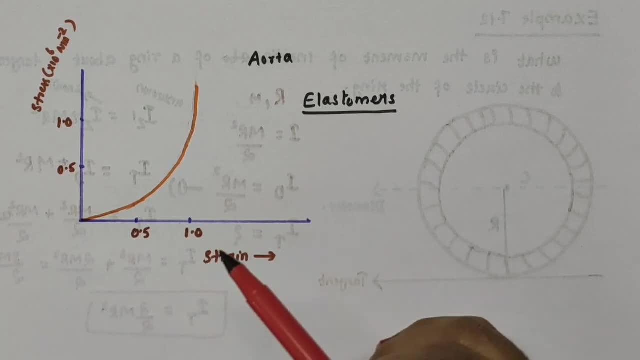 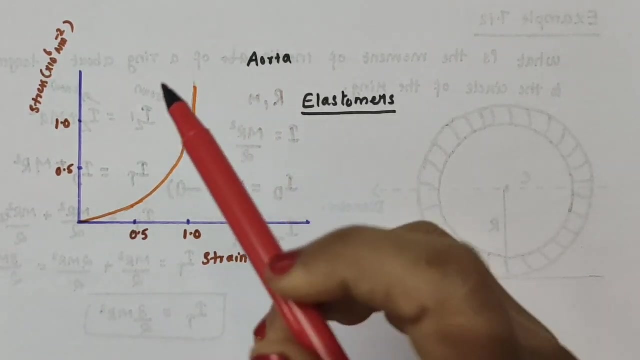 See the stress-strain behavior varies from material to material. This figure actually shows the stress-strain curve for the elastic tissue of aorta, Which is the large tube carrying blood from the heart. It is very clear from the graph that this material, that is, this tissue, does not obey Hooke's law. 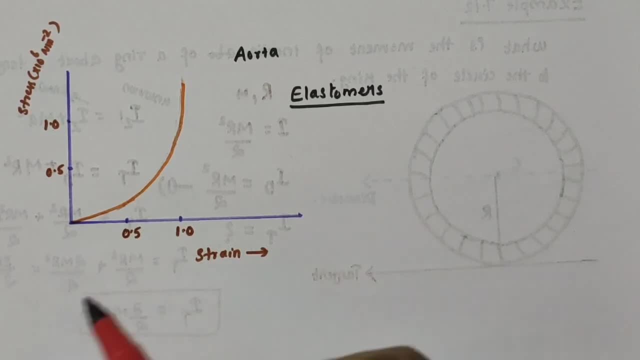 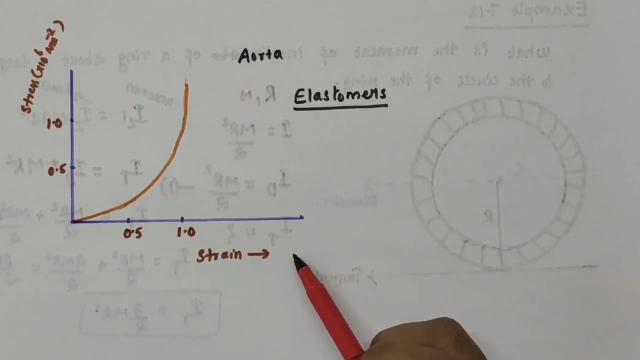 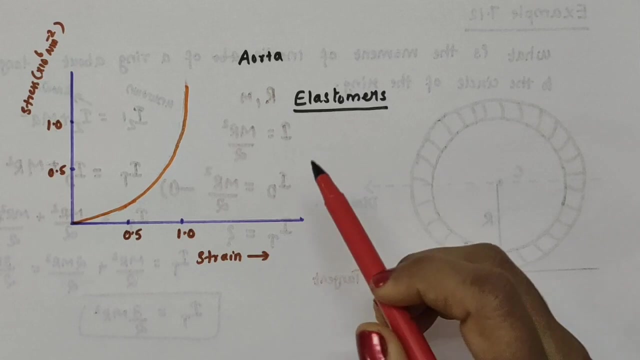 But its elastic region is very large and there is no well-defined plastic region for this material. Substances like rubber, tissue of aorta etc. which can be stretched to cause large strains, are called as elastomers. See, rubber can be stretched to cause large strains are called as elastomers. 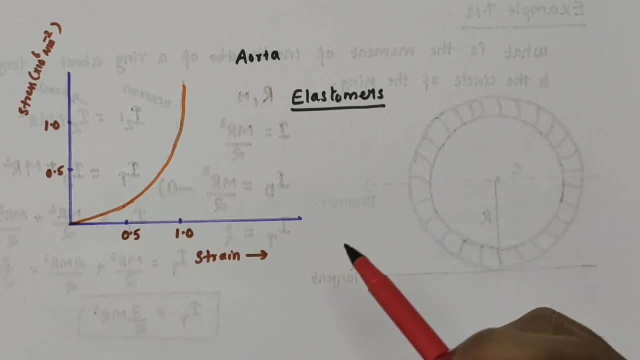 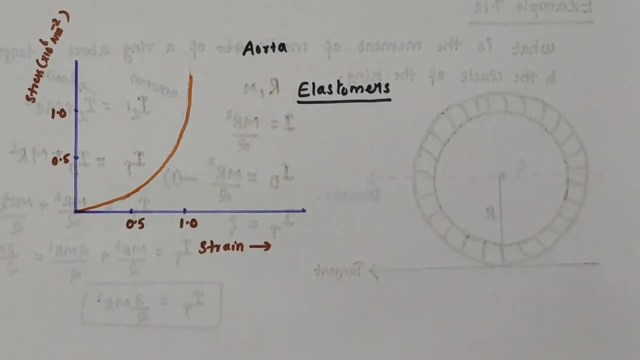 See, rubber can be stretched to cause large strains- are called as elastomers. Rubber can be pulled to several times its original length and still returns to its original shape. So elastomers are materials exhibiting elastic-like properties or rubber-like properties. So in this video we have discussed about stress-strain curve.